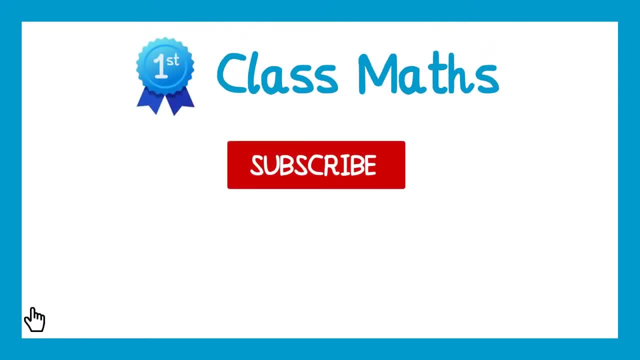 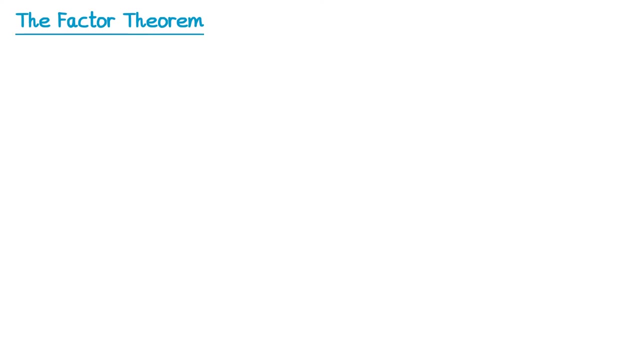 In this video we're going to learn about the factor theorem. As usual, there are some exam questions in the video's description that you can try afterwards. Let's start with a quadratic equation. In order to solve this, most people would probably factorise. You can factorise. 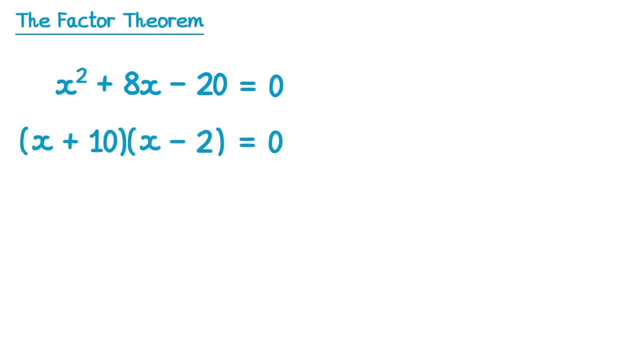 the left hand side as x plus 10, x minus 2.. These two brackets here are known as factors. They're factors since they multiply to give you the quadratic. If we then said we'll look at this first bracket, x plus 10, if that's going to equal 0, then we get the solution. 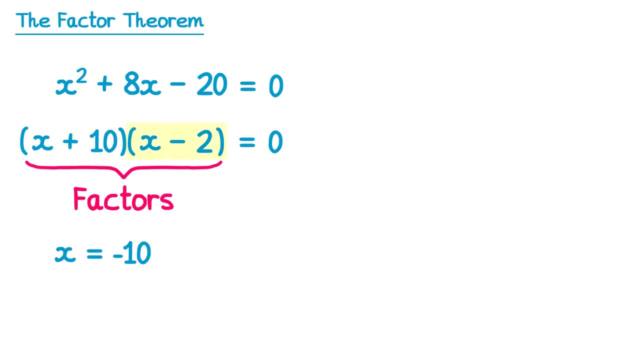 x equals negative 10, and the second bracket, x minus 2 equals 0. that will give us x equals 2.. These are both known as solutions. The reason they're solutions is if you substitute either of them back into the original quadratic here, you will get 0. Let's just verify that. 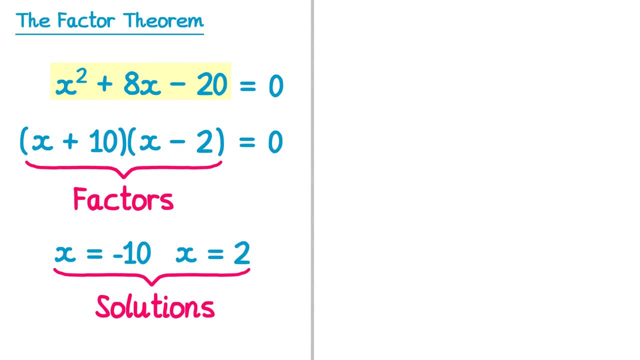 that's true. So if we substitute negative 10 in, we do negative 10 squared plus 8, lots of negative 10 take 20.. Negative 10 squared is 100.. 8 times negative 10 is negative 80, and then take away 20.. And this does indeed give 0.. And what about 2?? So if we substitute 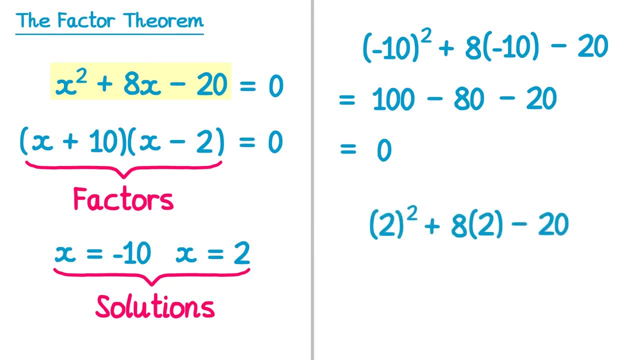 2 in 2 squared plus 8 lots of 2, take 20.. 2 squared as 4,, 8 lots of 2 is 16, and then take 20.. And again, this does give 0.. So the reason: 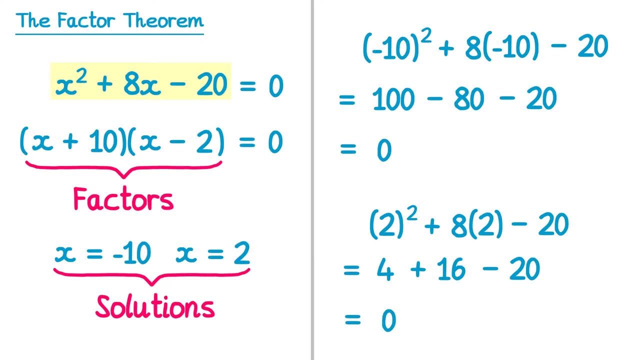 they're solutions is because if you substitute them in, they do give you 0.. Now the factor theorem is concerned with the link between the solutions and the factors. If you look at this solution here, x equals negative 10, that corresponds to a factor. 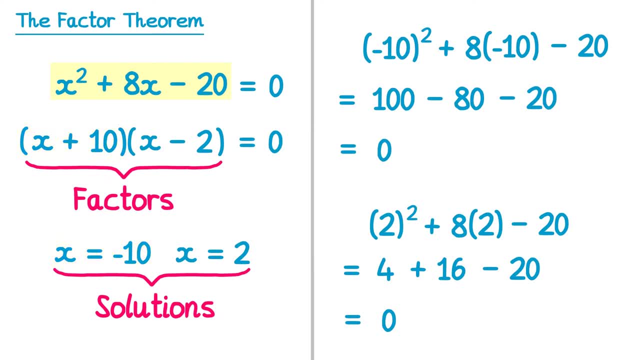 of x plus 10.. And if you see this solution here, x equals 2, this corresponds to a factor of x minus 2.. So if you know the solutions, you can also find the factors just by doing x and then doing the opposite sign of the solution. So when it's positive you do negative. 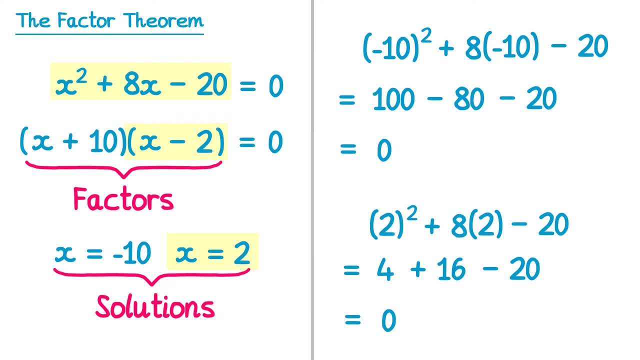 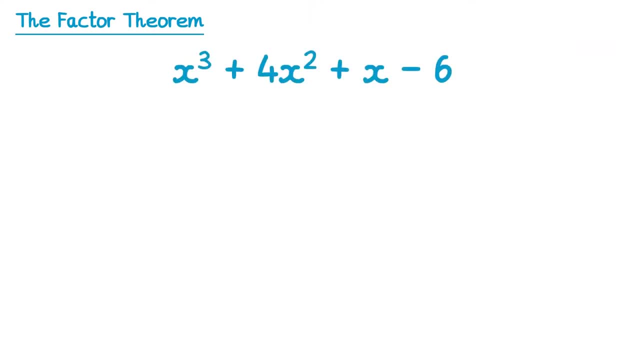 and when it's negative, you do positive. Let's have a look at this with an example. Now let's look at this cubic expression. here I'm going to substitute in some numbers. If I substitute in a number and I get 0 as the result, then I know I've found a factor. 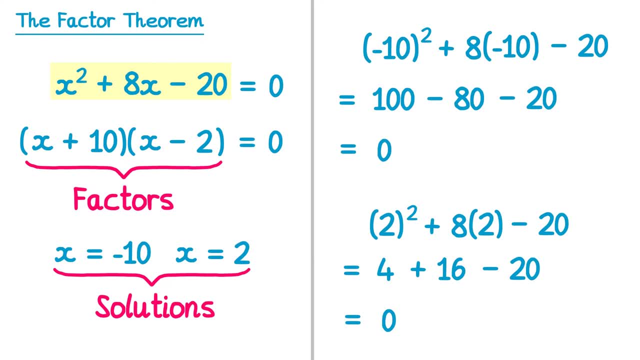 the reason they're solutions is because if you substitute them in, they do give you 0.. Now the factor theorem is concerned with the link between the solutions and the factors. If you look at this solution here: x equals negative 10, that corresponds to a factor of x plus 10.. And if you see this solution here, x. 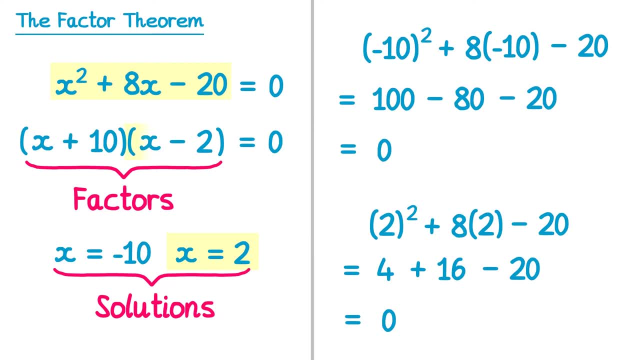 equals 2,. this corresponds to a factor of x minus 2.. So if you know the solutions, you can also find the factors just by doing x and then doing the opposite sign of the solution. So when it's positive you do negative, and when 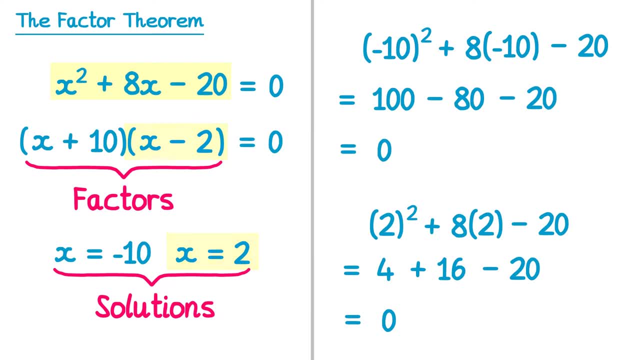 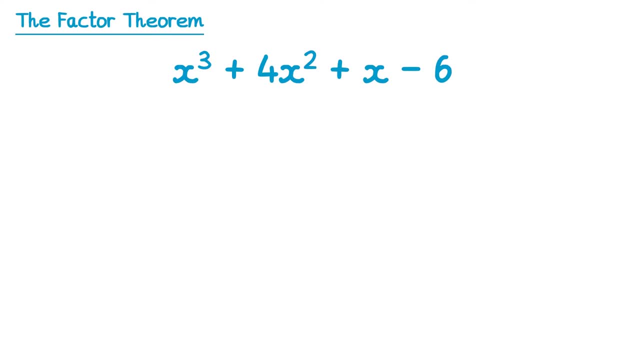 it's negative, you do positive. Let's have a look at this with an example. Now let's look at this cubic expression. here I'm going to substitute in some numbers. If I substitute in a number and I get 0 as the result, then I know I. 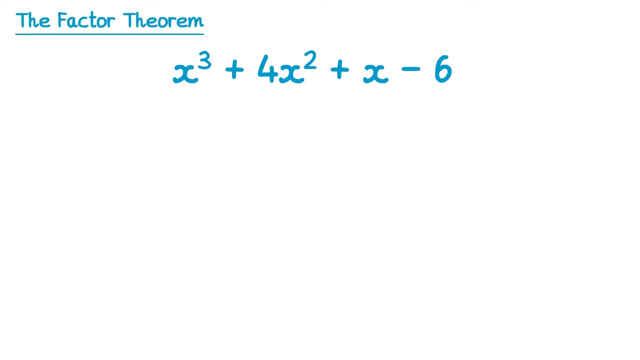 found a factor. I'm going to start with the number 1.. So 1 cubed plus 4, lots of 1 squared plus 1, takes 6.. 1 cubed is just 1.. 4- lots of 1 squared. well, 1 squared is 1 and times 4,. 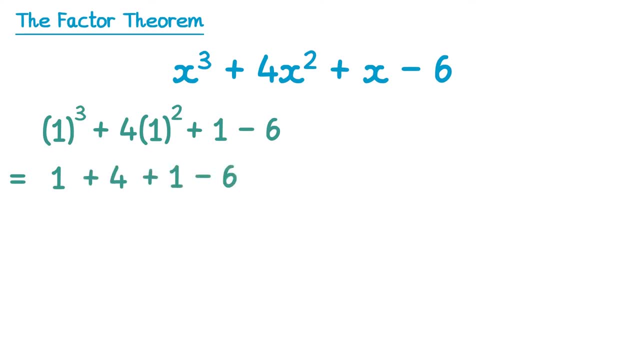 that gives 4, and then we've got plus 1 takes 6.. 1 add 4, add 1 is 6, so 6 takes 6 does give you 0.. Now I substituted in here a positive 1. This means that my 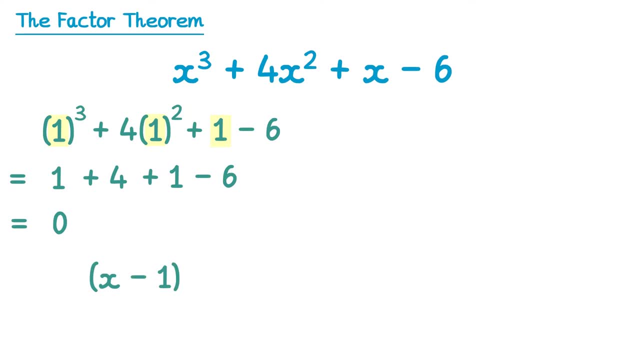 factor will be equal to 0. So if I substitute in here a positive 1, this means that my factor will be x take away 1.. So x take away 1 is a factor. Let's try a different number This time. we'll do negative 4.. So negative 4. cubed plus 4, lots of. 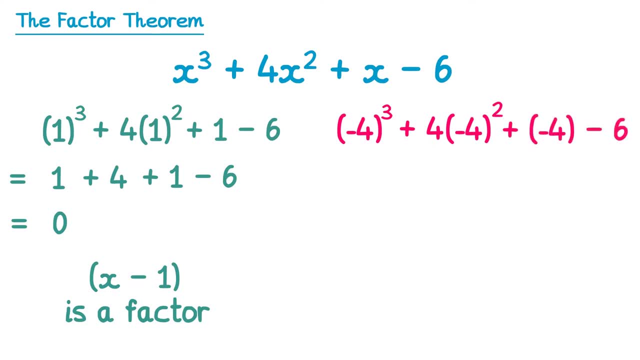 negative 4 squared plus negative 4 takes 6.. Negative 4 cubed is negative 64, then we've got 4 lots of negative 4 squared. Well, negative 4 squared is positive 16, and 4 lots of 16 is 64,, so plus 64. Then we've got take 4, takes 6.. 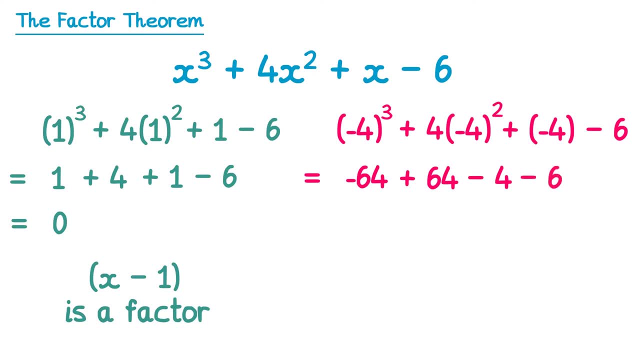 And if you simplify this well, the 64s there will cancel out. so it's negative. 4 takes 6, which is negative 10.. Now this doesn't come out as 0. So since we substituted in negative 4 here, then the bracket we were considering was actually x plus 4.. But since 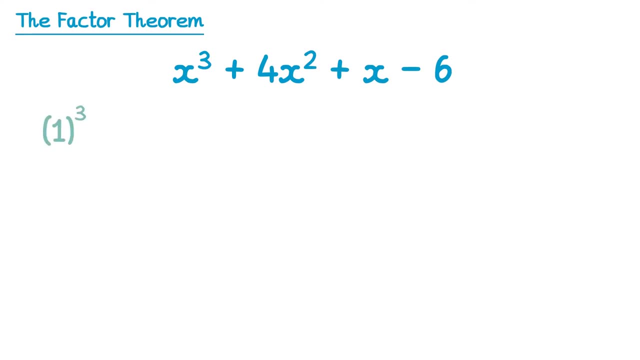 I'm going to start with the number 1.. So 1 cubed plus 4, lots of 1 squared plus 1, takes 6.. 1 cubed is just 1.. 4, lots of 1 squared. well, 1 squared is 1, and times 4, that gives 4.. And then we've got plus 1 takes. 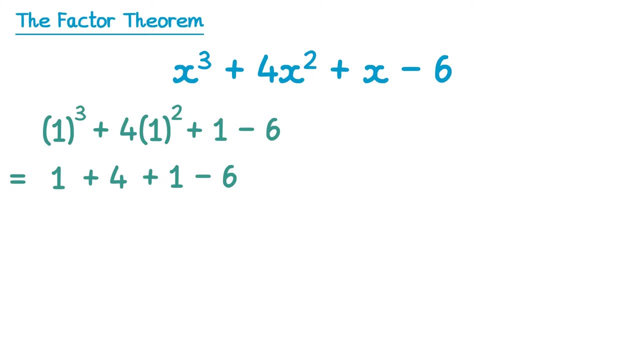 6.. 1 add 4. add 1 is 6, so 6 takes 6 does give you 0.. Now I've substituted in here a positive 1.. This means that my factor will be x, take away 1.. 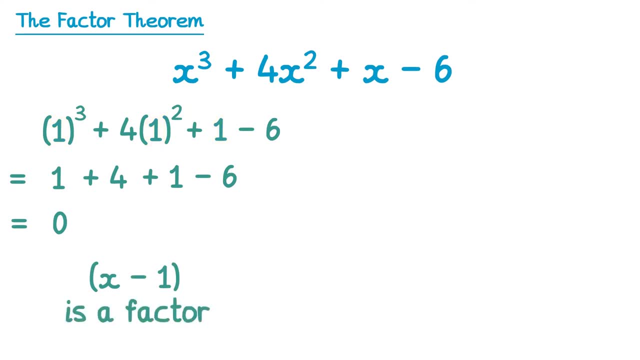 x. take away, 1 is a factor. Let's try a different number This time. we'll do negative 4.. So negative 4 cubed plus 4, lots of negative 4 squared plus negative 4 takes 6.. Negative 4 cubed is negative 64. Then we've got 4, lots of negative 4 squared. Well, negative 4 squared. 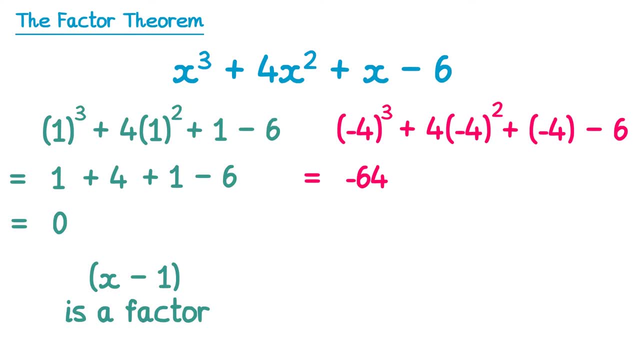 is positive: 16 and 4. lots of 16 is 64, so plus 64. Then we've got: take 4 takes 6. And if you simplify this well, the 64s there will cancel out. so it's negative: 4 takes 6, which. 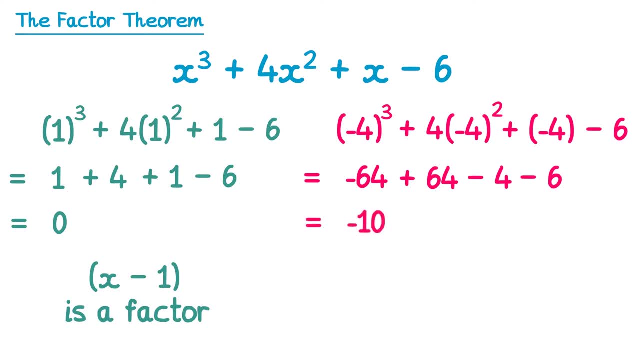 is negative 10.. Now this doesn't come out as 0. So since we substituted in negative 4 here, then the bracket we were considering was actually x plus 4.. But since this doesn't give 0, it gives negative 10. then unfortunately this is not a factor. 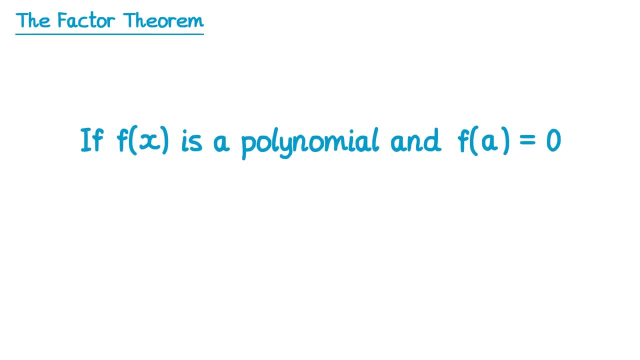 So the factor theorem states that if f of x is a polynomial and f of a equals 0, so a was the number we were substituting in then. x minus a is a factor of f of x. Let's have a look at how questions can be written in exams. Show that x plus 5 is a. 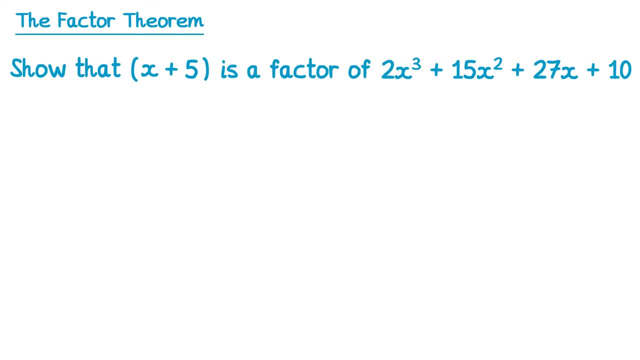 factor of this? So the factor in this question is x plus 5.. This means that if we do the opposite sign so negative 5 and substitute that in, we need to get 0. So if we do f of negative 5, this will be 2, lots of negative 5, cubed plus. 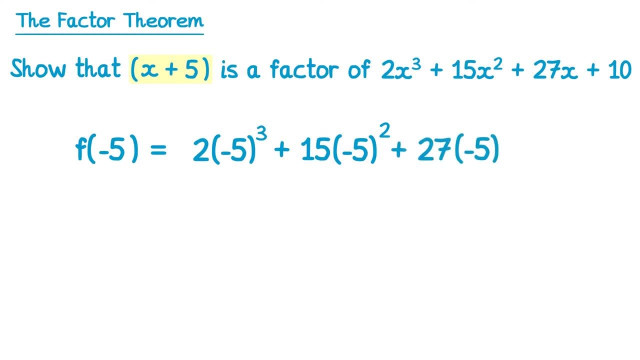 15. lots of negative, 5 squared plus 27. lots of negative 5 plus 10.. Now, because this is a show that question. you really need to show all of the steps. You can't just type this into your calculator and write equal 0. So negative 5 cubed is negative 125 and 2 lots. 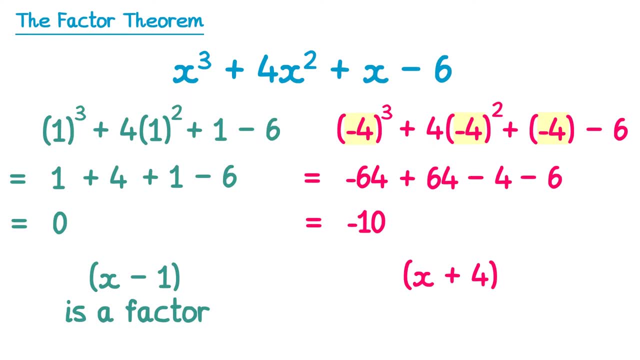 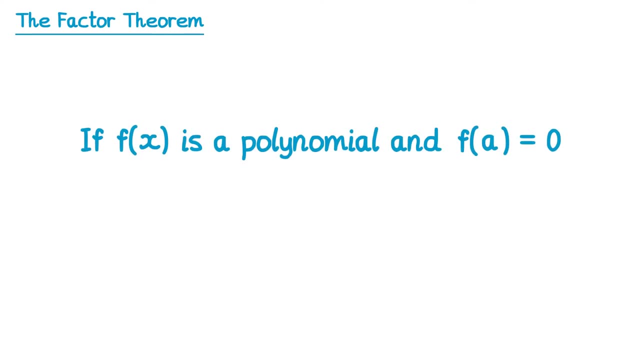 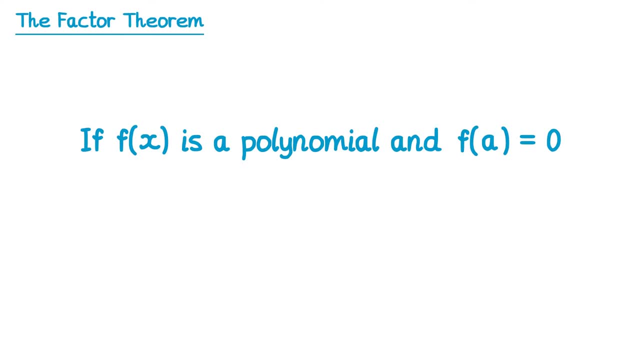 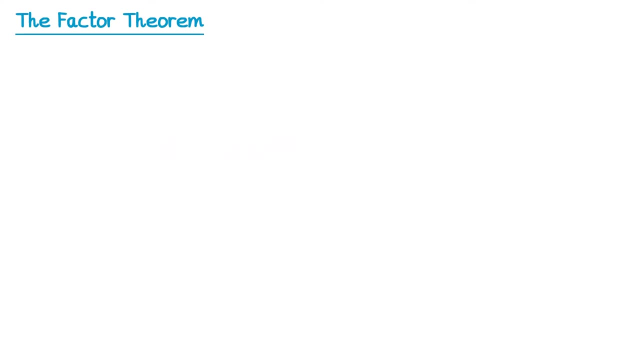 What's news in this section? Let's have a look at how questions can be written in. exams Show that x plus 5 is a factor of this. So the factor in this question is x plus 5.. This means that if we do the opposite, sign so negative 5, and substitute 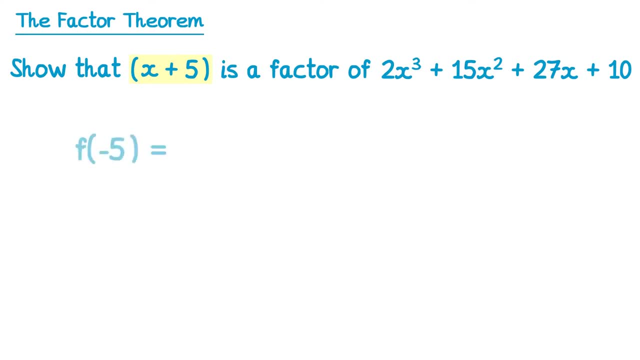 that in we need to get 0.. So if we do f of negative 5, this will be 2, lots of negative 5 cubed plus 15. lots of negative 5 squared plus 27. lots of negative 5, plus 10.. Now, because this. 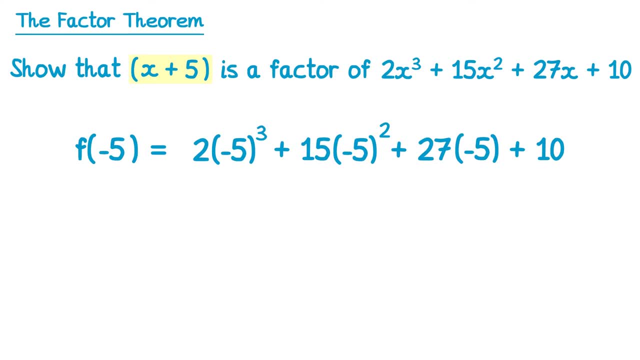 is a show that question. you really need to show all of the steps. You can't just type this into your calculator and write equal 0.. So negative 5 cubed is negative 125 and 2 lots of that is negative 250.. Negative 5 squared is 25 and 15- lots of 25 will give you plus 375.. 27- lots of negative. 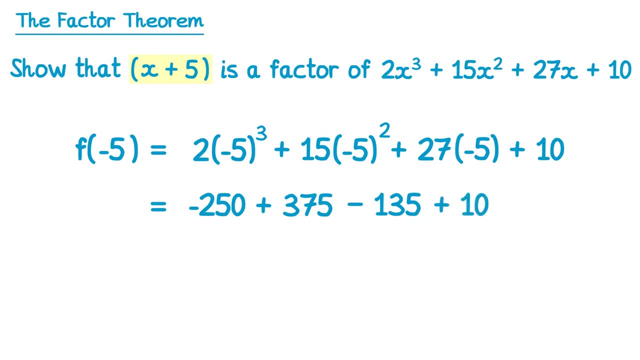 5 is. take 135 and then plus 10.. Now at this point you can show that that does indeed equal 0. So we've managed to show that f of negative 5 does give you 0, so x plus 5 is a factor. 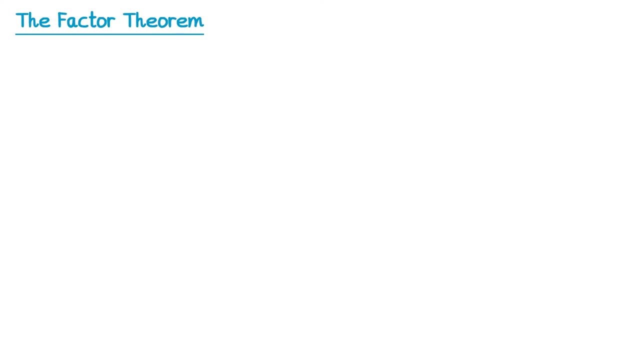 The factor theorem can be especially useful when you're trying to factorize polynomials. Let's imagine we had to factorize this cubic here. We know now that if we substitute in a number and we get 0 out, then we found one of the factors. 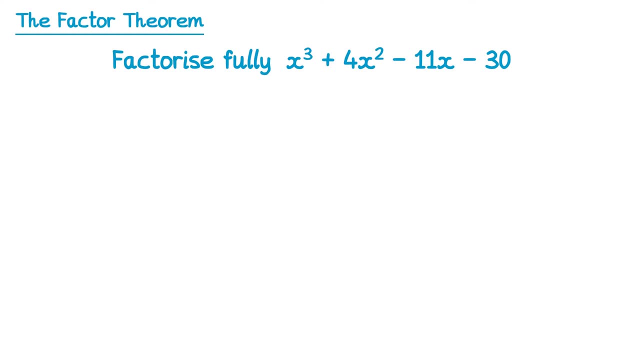 The only question is how to do that. The only question is: which number do you choose to substitute? Well, in your exam, you'll probably be given one of the factors. If you aren't, though, then you want to look at the last term here. 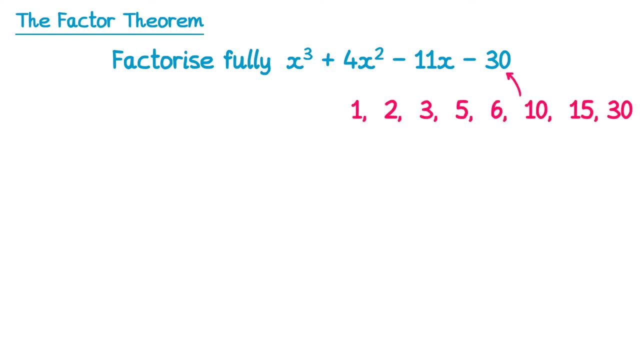 Look at the factors of 30. So 1,, 2,, 3,, 5,, 6,, 10,, 15 and 30, and also the negatives of those. These would be the numbers to try. Now, there's an awful lot of numbers here, obviously. 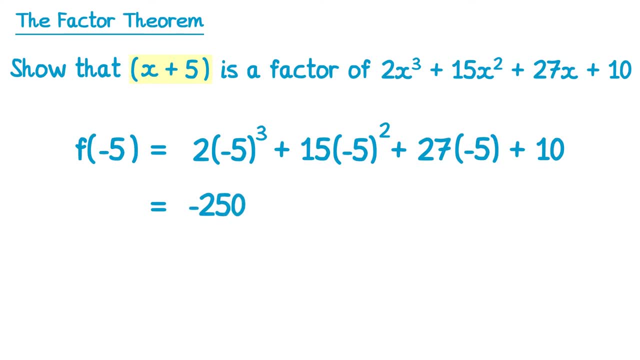 of that is negative 250.. Negative 5 squared is 25 and 15. lots of 25 will give you plus 375.. 27, lots of negative 5 is take 135.. and then plus 10.. Now, at this point you can show that that does indeed equal 0.. 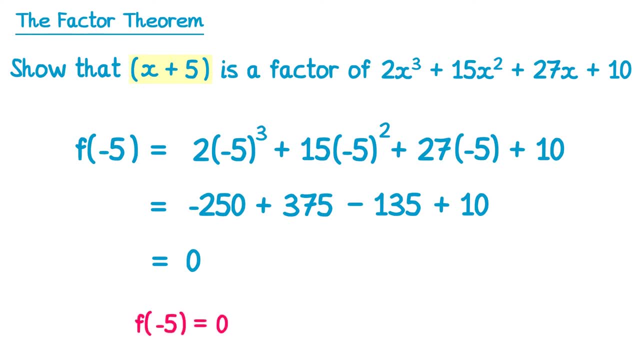 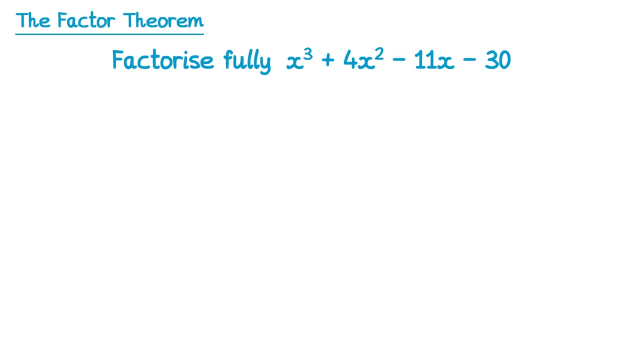 So we've managed to show that f of negative 5 does give you 0,. so x plus 5 is a factor. The factor theorem can be especially useful when you're trying to factorise polynomials. Let's imagine we had to factorise this cubic here. We know now that if we substitute in 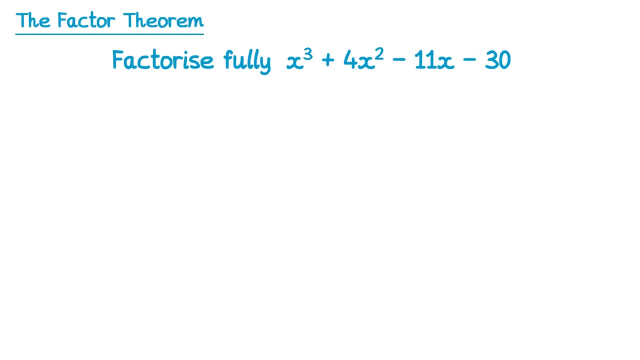 a number and we get 0 out, then we've found one of the factors. The only question is: which number do you choose to substitute? Well, in your exam, you'll probably be given one of the factors. If you aren't, though, then you want to look at the last term here. Look at: 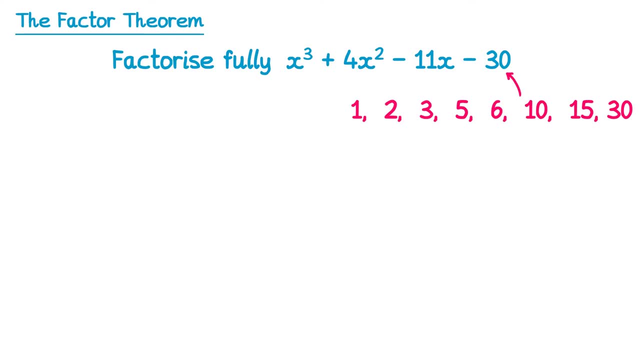 the factors of 30,, so 1,, 2,, 3,, 5,, 6,, 10,, 15 and 30, and also the negatives of those. These would be the numbers to try. Now, there's an awful lot of numbers here, obviously, so I'm 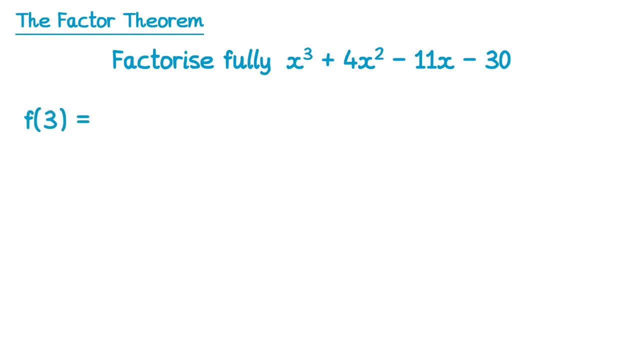 going to choose one that I know is a factor. I'm going to do f of 3.. f of 3 is 3 cubed plus 4 lots of 3 squared. Take 11, lots of 3, and take 30.. 3 cubed is 27,, 3 squared is 9, and times that by 4 is 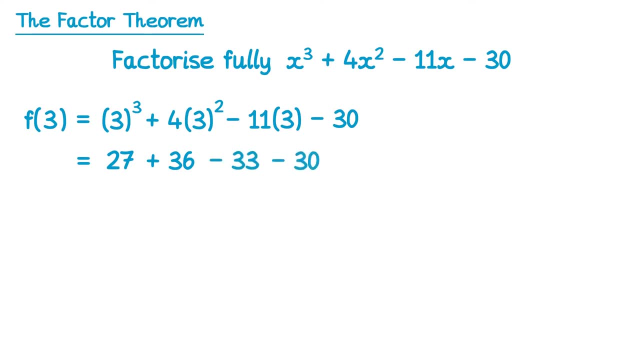 36. Negative 11 times 3 is negative 33, and then take 30. And this does give you 0. So we've substituted in positive 3, in which case x take 3 is a factor. Now we could continue this method to try and find the other factors just by guessing numbers. 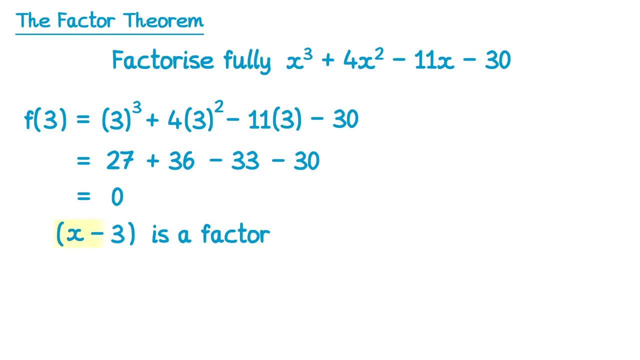 or there is a quicker way: Now that we have one of the factors x, take away 3, we can divide this into the original polynomial and see what we get using polynomial long division. So let's do that now. So we'll do a bus stop, Put the cubic inside and the linear factor we've just found outside. 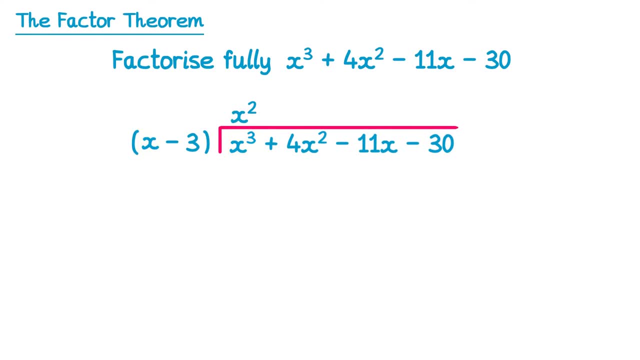 We'll do x cubed divided by x, which gets you x squared. Multiply that back through x squared times. x is x cubed. x squared times negative 3, negative 3x squared. Then subtract these x cubed. take x cubed is 0.. 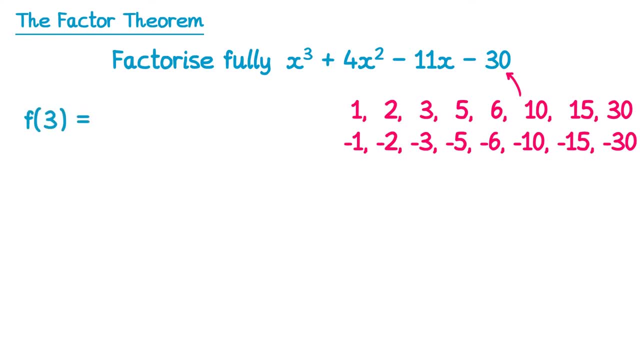 so I'm going to choose one that I know is a factor. I'm going to do f of 3.. f of 3 is 3 cubed plus 4.. So I'm going to do f of 3 squared. take 11, lots of 3, and take 30.. 3 cubed is 27.. 3 squared is 9 and 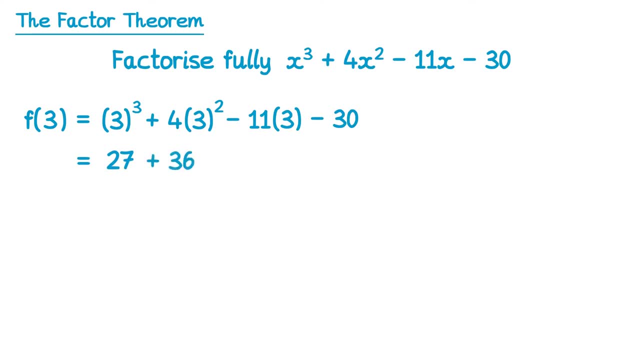 times that by 4 is 36.. Negative 11 times 3 is negative 33, and then take 30. And this does give you 0. So we've substituted in positive 3, in which case x take 3 is a factor. Now we could continue. 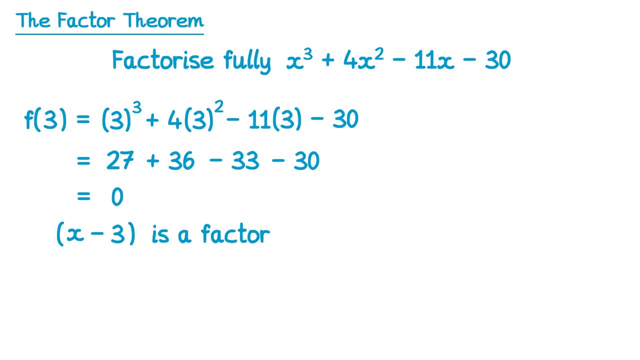 this method to try and find the other factors just by guessing numbers. or there is a quicker way, Now that we have one of the factors: x, take away 3, we can do f of 3.. So we can do f of 3,. x take 3,. 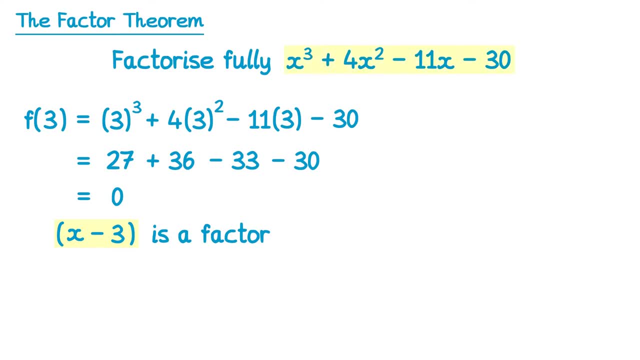 we could divide this into the original polynomial and see what we get using polynomial long division. So let's do that now. So we'll do a bus stop, put the cubic inside and the linear factor we've just found outside. We'll do x cubed divided by x, which gets you x squared. Multiply that back through. 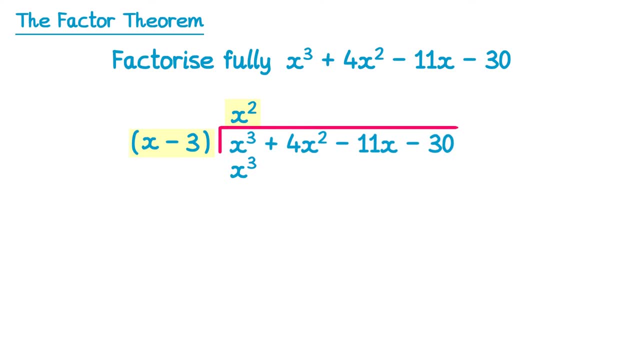 x squared times. x is x cubed. x squared times: negative: 3, negative: 3x squared. Then subtract these: x cubed. take x. cubed is 0.. f squared is negative. 10x squared plus 2x x squared. take x and multiply by x x squared. 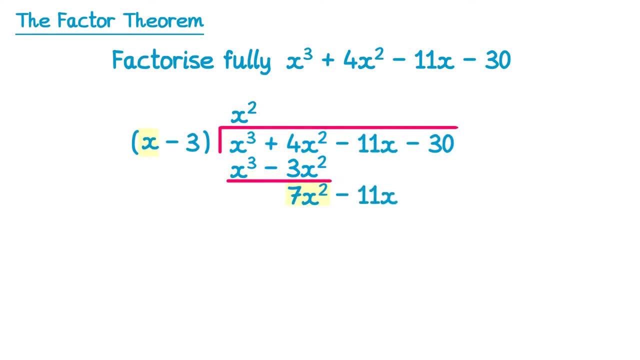 4x squared. take away negative: 3x squared is 7x squared. then bring down the next term. Do 7x squared divide by x, which is plus 7x. Then multiply that plus 7x back through 7x times x is 7x squared. 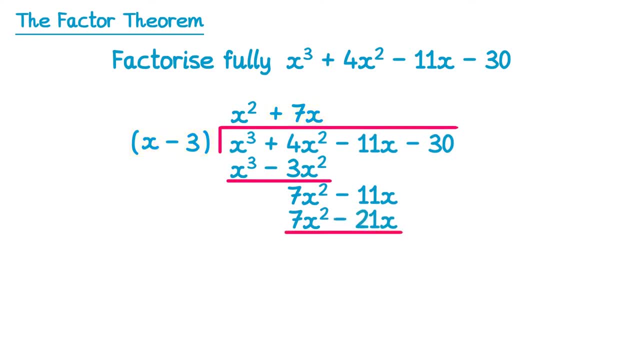 7x times negative 3 negative 21x. Then we subtract The 7x squared will cancel Negative 11x. take away negative 21x is 10x. Then bring down the final term. Do 10x squared divide by x, which is 7x squared, Then subtract those. 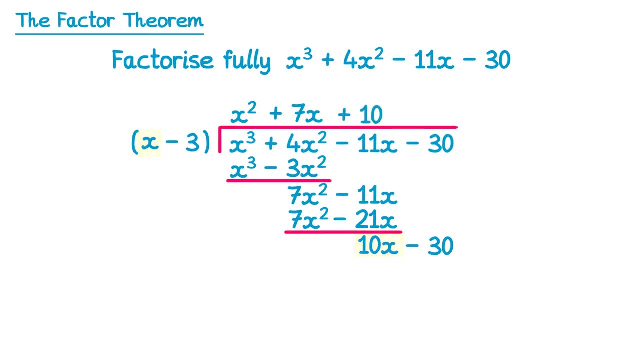 Do 10x divided by x, which is plus 10, and then multiply that plus 10 back through, So 10 times x, 10x and 10 times negative 3, negative 30. And if you subtract these you get 0. 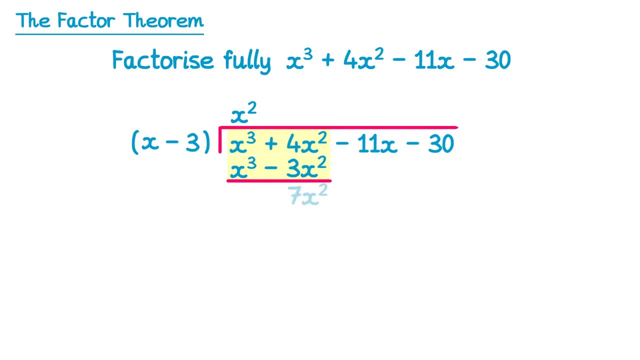 4x squared. take away negative 3x squared is 7x squared. Then bring down the next term. Do 7x squared divide by x, which is plus 7x. then multiply that plus 7x back through 7x times x. is 7x squared, 7x times negative 3, negative 21x. then we subtract. 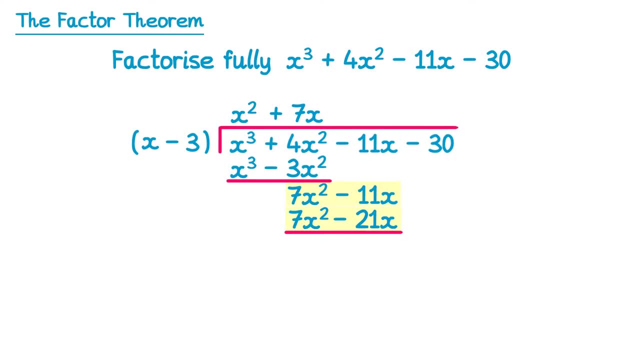 The 7x squareds will cancel negative 11x. take away negative 21x is 10x. Then bring down the final term, Do 10x squared, divide by x, which is plus 10, and then multiply that plus 10 back through. 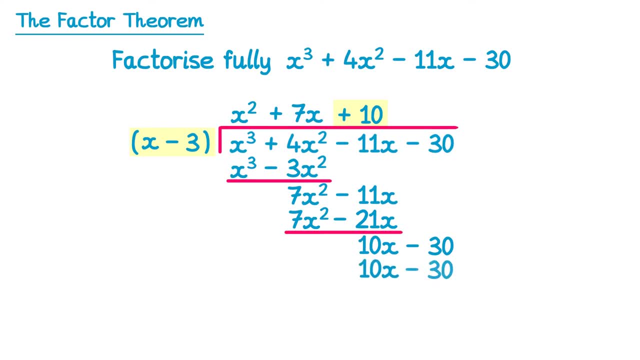 So 10 times x is 10x and 10 times negative 3 is negative 30, and if you subtract these you get 0. So if you divide this cubic by this linear term here, you end up with this quadratic term. 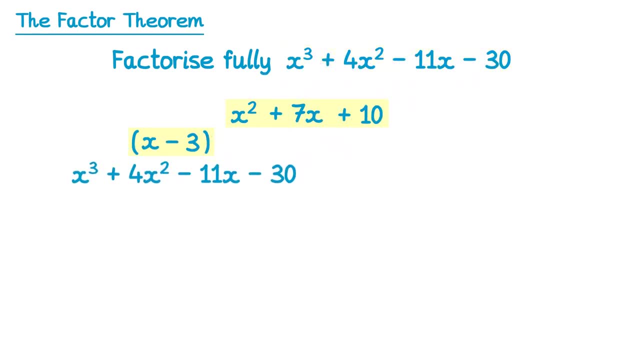 That means that this cubic is equal to the product of the linear term and the quadratic term. So we're nearly there. We've managed to factorise this into a linear term and a quadratic term, But this quadratic term also factorises itself, So this is equal to the linear term, and if you factorise this quadratic term, you'll get 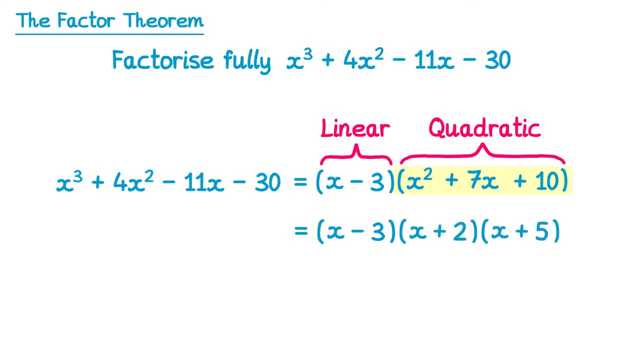 x plus 2 and x plus 5.. So we've now managed to fully factorise the cubic using the factor theorem first and then polynomial long division. You could also be asked to solve cubic equations. So if we were asked to solve cubic equations, we could do this. 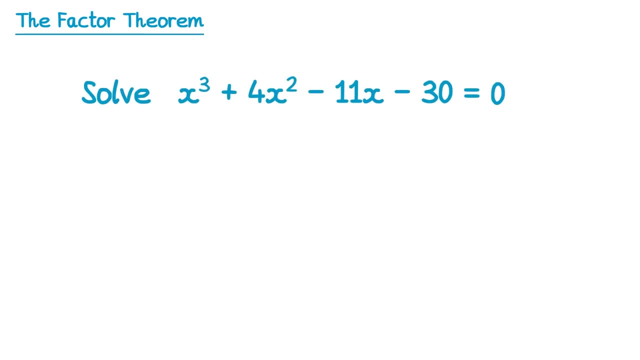 If we were asked to solve this cubic equation- notice, it's the same as the last one, but it's now an equation because it has equals 0, we would factorise it like we just did and then we would find our solutions. So from the bracket we get the solution: x equals 3, the bracket gives x equals. 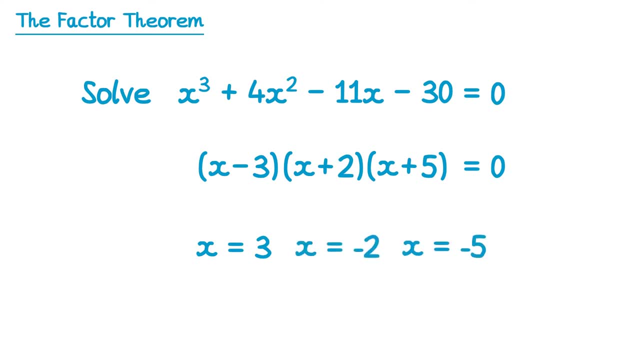 negative 2, and the bracket gives x equals negative 5.. Now there's one more type of question you need to be aware of. Imagine: we were asked to show that this bracket was a factor of this cubic. Now, if you look at this factor here, you'd probably say, well, we've got plus 1, so we'll. 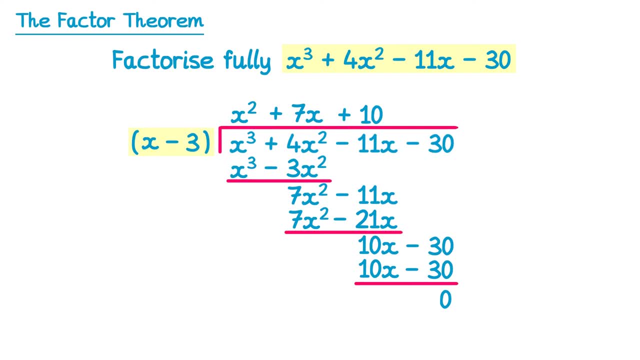 So if you divide this cubic by this linear term, here you end up with this quadratic term. That means that this cubic is equal to the product of the linear term and the quadratic term. So we're nearly there: We've managed to factorise this into a linear term and a quadratic term. 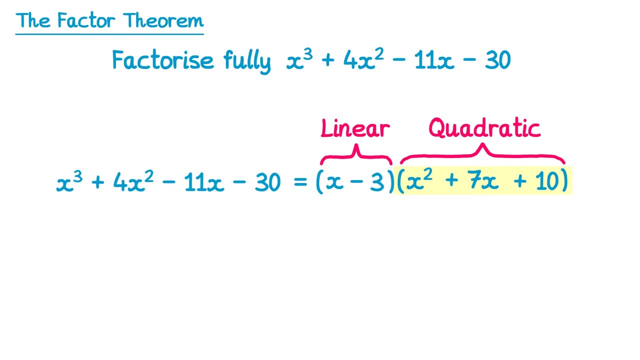 But this quadratic term also factorises itself. So this is equal to the linear term, and if you factorise this quadratic term you'll get x plus 2 and x plus 5.. So we've now managed to fully factorise the cubic using the factor theorem first, and 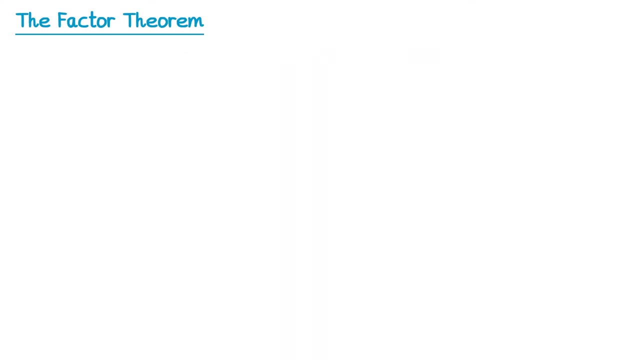 then polynomial long division. You could also be asked to solve cubics. Let's see how each one actually solves the cubic equations. So if you were asked to solve this cubic equation, Notice it's the same as the last one And because the equation has equals 0, we would factorise it like we just did. 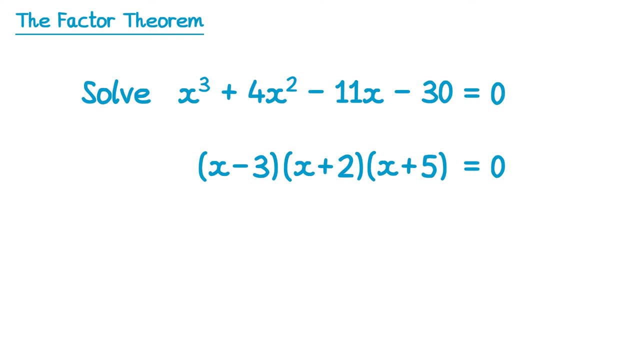 And then we would find our solutions. So from the x minus 3 bracket we get the solution x equals 3, the x plus 2 bracket gives x equals negative 2 and the x plus 5 bracket gives x equals negative 5.. 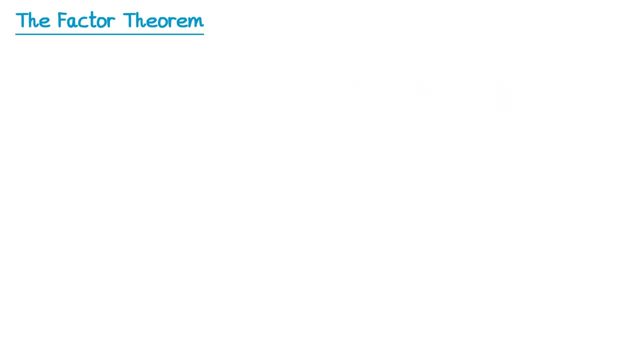 Now there's one more type of question you need to be aware of. Hear, hear, Imagine we were asked to show that this Taylor zum Becker became products. log of x plus 2 braket times x equals negative 5. We get those two пример abstracts to become the keeprank for our analysis. 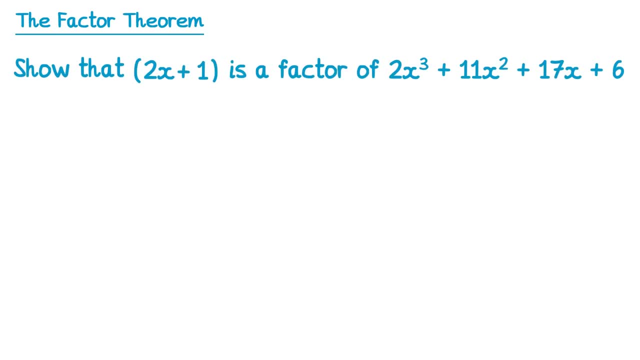 5,, 6 and 2.. This is where the alphabet organizizes our laws. x plus 1 was a factor of this cubic. Now, if you look at this factor here, you'd probably say, well, we've got plus 1, so we'll do the opposite. sign negative 1. and if we substitute a negative 1, 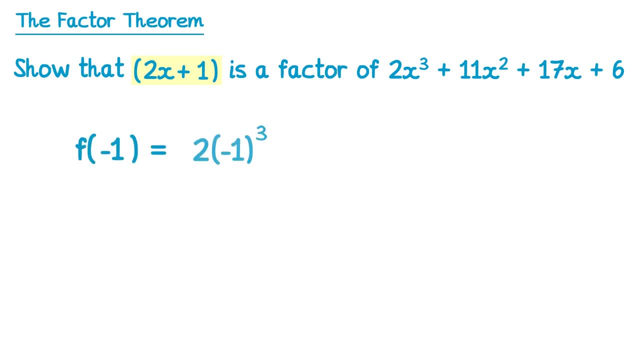 we'll get 0.. So you'd do f of negative 1, which is 2 lots of negative 1 cubed plus 11. lots of negative 1 squared plus 17. lots of negative 1 plus 6.. 2 lots of negative 1 cubed is negative 2,. 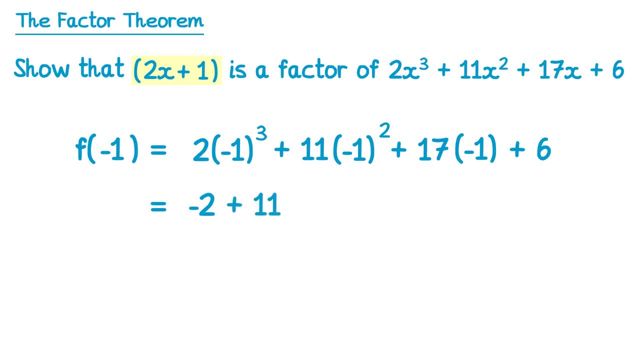 11. lots of negative 1, squared is just 11 and 17. lots of negative. 1 is negative 17 and then plus 6.. Now, if you do this, you end up with negative 2, not 0 like you expected, but 2x plus 1 is actually. 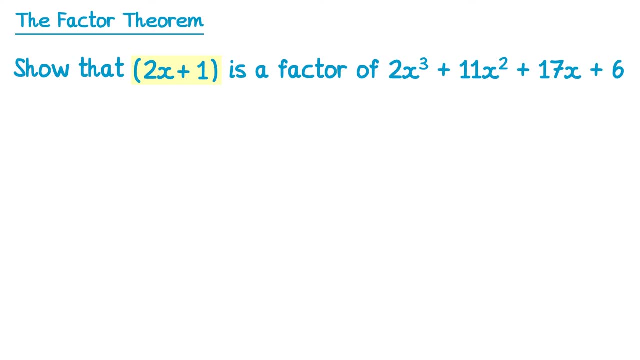 do the opposite: sign negative 1, and if we substitute a negative 1 we'll get 0. So you'd do f of negative 1, which is 2 lots of negative, 1 cubed, plus 11 lots of negative. 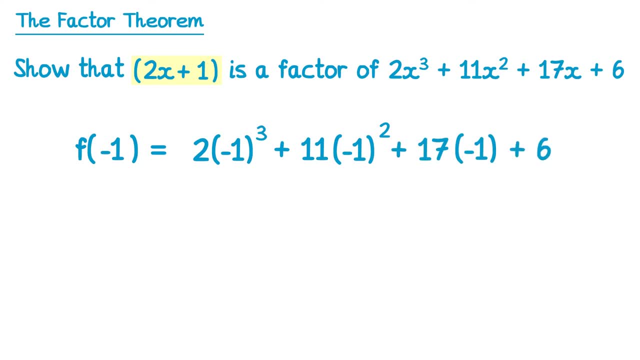 1 squared plus 17. lots of negative 1, plus 6.. 2- lots of negative. 1 cubed is negative 2, 11- lots of negative. 1 squared is just 11, and 17: lots of negative. 1 is negative 17,, and then plus 6.. 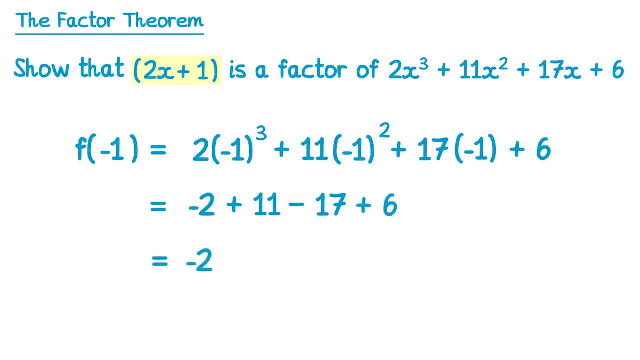 Now, if you do this, you end up with negative 2, not 0 like you expected, but 2x plus 1 is actually a factor of this cubic, so something else is going on. The difference here is this number 2.. 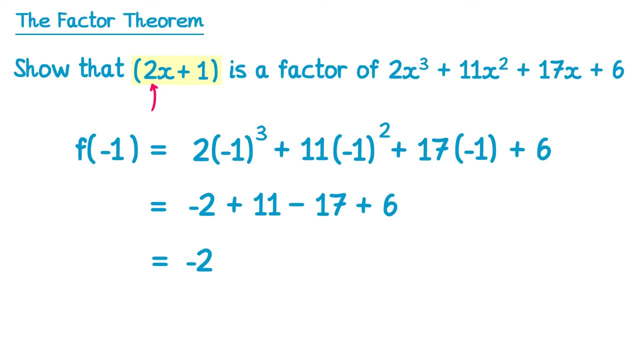 This wasn't there for any of the other factors, So the number we substitute in isn't actually negative 1.. What you want to do is take this bracket- 2x plus 1, and set it equal to 0. If we take 1 from both sides, we get 2x equals negative 1.. 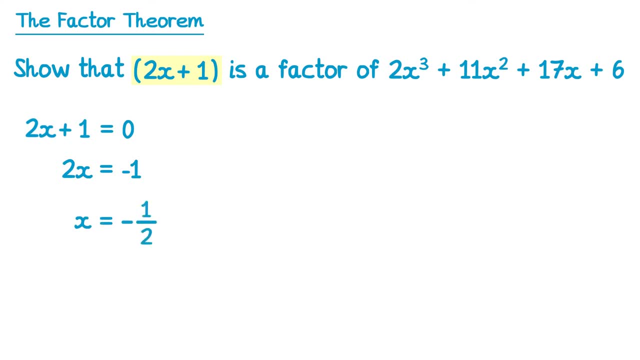 And then divide both sides by 2. We get x equals negative 1 half. So this would be the solution if this were an equation, In which case negative 1 half is what we actually need to substitute in. So if you do f of negative 1 half, you do 2 lots of negative 1 half cubed plus 11 lots. 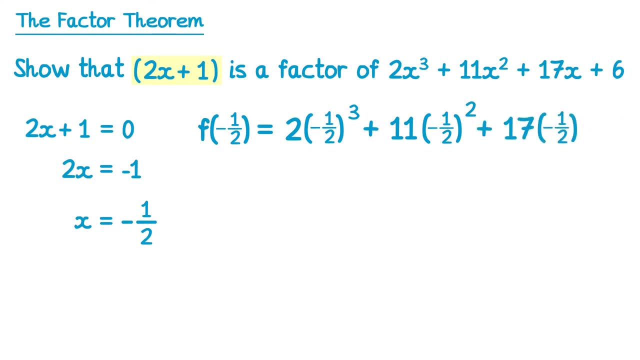 of negative 1 half squared plus 17. lots of negative 1 half plus 6.. If we do negative 1 half cubed we get negative 1- eighth. so 2, lots of negative 1 eighth. Negative 1 half squared is a positive quarter. 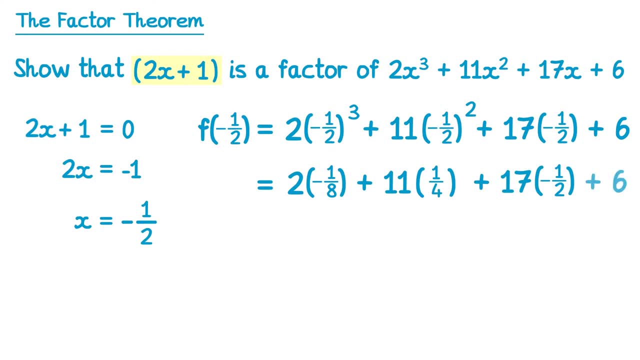 That's 11 quarters plus 17. lots of negative 1 half plus 6.. Now, if we do 2, lots of negative 1. eighth, we end up with negative 2 over 8, which simplifies to negative 1 quarter. 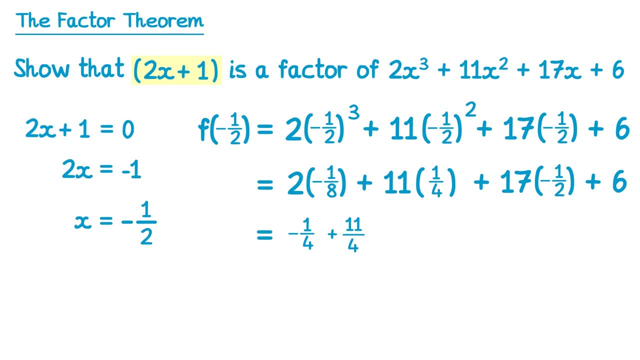 Now we'll do 11 quarters. Then we've got 17 times negative 1 half, which is negative 17 over 2, and then plus 6.. Now, to make this easy, we'll write all of these over 4.. So for the final two terms, we've got negative 17 over 2, which is the same as negative 34. 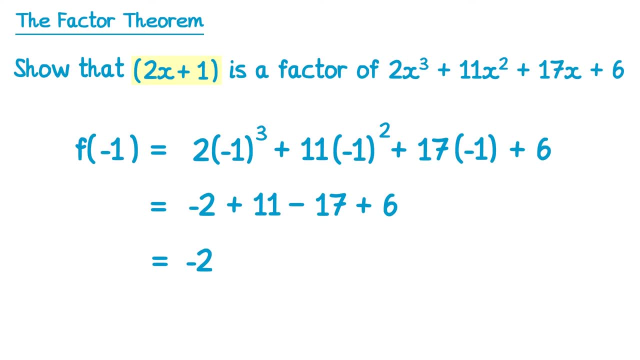 a factor of this cubic, so something else is going on. The difference here is this number 2.. This wasn't there for any of the other factors, so the number we substitute in isn't actually negative 1.. What you want to do is take this bracket. 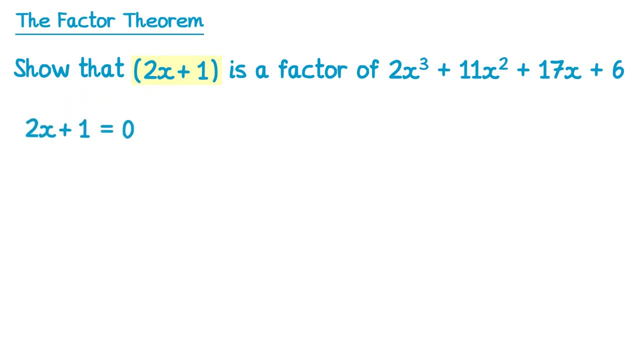 and set it equal to 0.. If we take 1 from both sides, we get 2x equals negative 1, and then divide both sides by 2, we get x equals negative 1 half. So this would be the solution if this were an equation, in which case negative 1 half is what we actually need to substitute in. 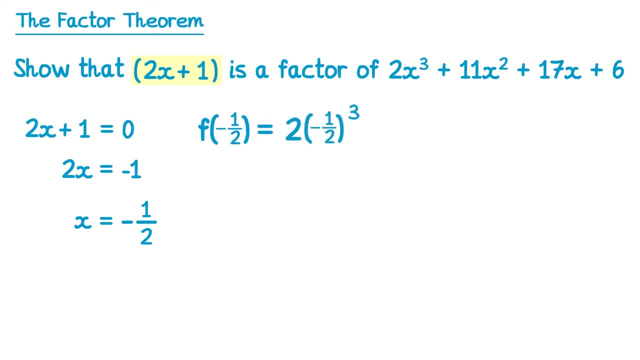 So if you do f of negative 1 half, you do 2 lots of negative 1 half cubed plus 11. lots of negative 1 half squared plus 17 lots of negative 1 half plus 6.. If we do negative 1 half cubed, 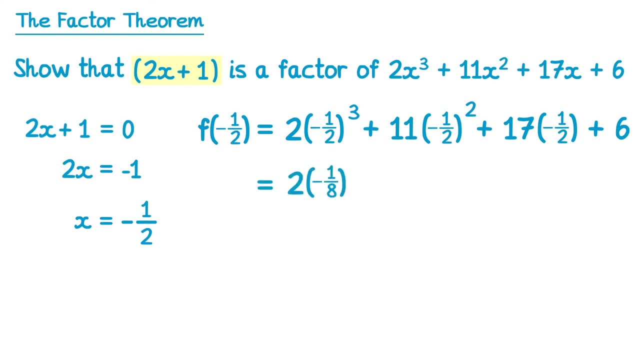 cubed, we get negative 1, eighth. so 2, lots of negative, 1, eighth. Negative 1, half squared is a positive quarter. so it's plus 11 quarters plus 17, lots of negative 1, half plus 6.. Now if we do 2, lots of negative 1, eighth. we end up with 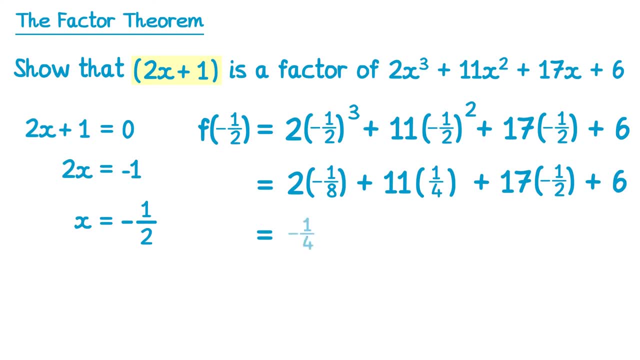 negative 2 over 8, which simplifies to negative 1 quarter. Now we'll do 11 quarters. then we've got 17 times negative 1 half, which is negative 17 over 2, and then plus 6.. Now, to make this easy, we'll write all of these over 4.. So 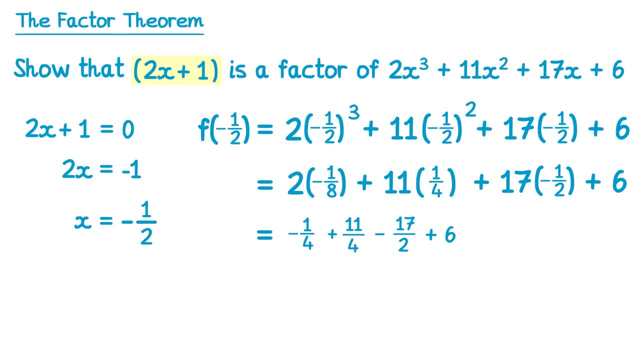 for the final two terms, we've got negative 17 over 2, which is the same as negative 34 over 4, and this positive 6 is the same as plus 24 over 4.. And if you do negative 1, add 11,, take 34, plus 24, you do indeed get 0.. So now we've shown. 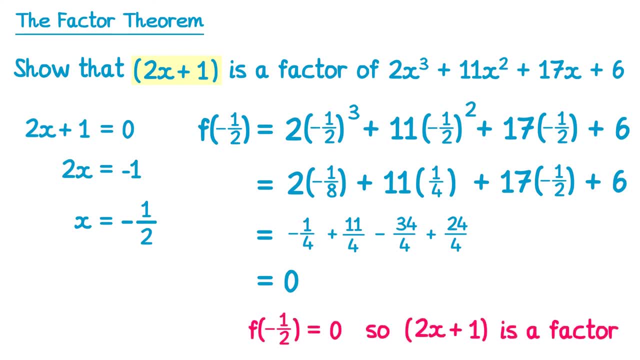 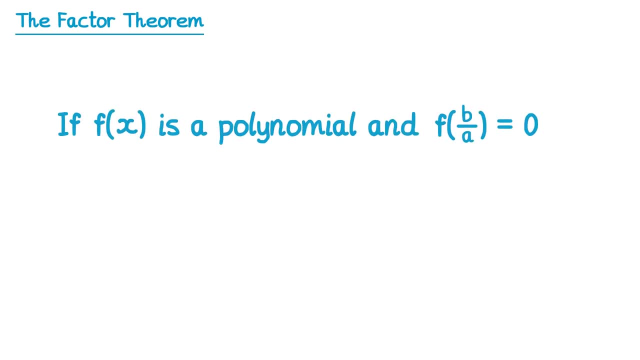 that f of negative 1 half equals 0, so the bracket 2x plus 1 is a factor. This means we need to slightly modify our factor theorem. So if f of x is a polynomial and f of b over a equals 0, then ax minus b is a factor of f of x. So 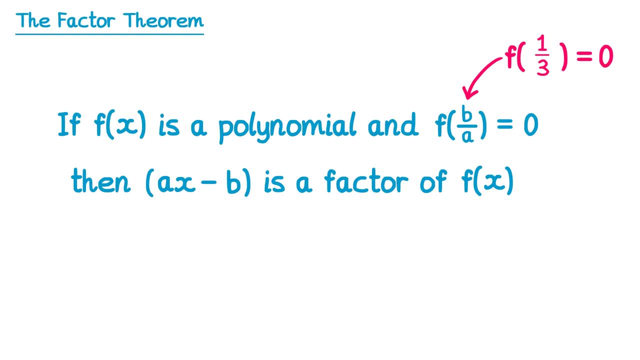 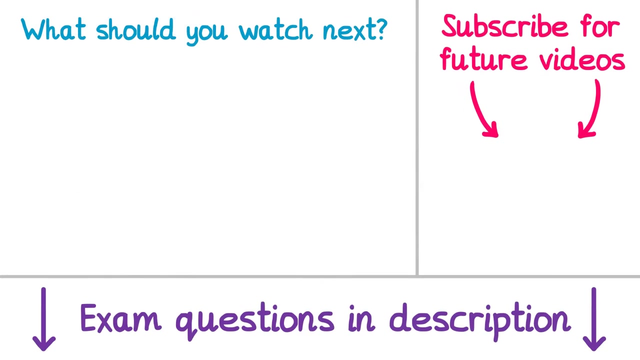 for example, if we had f of 1, third here, b is 1 and a is 3, so if we substitute that into the factor bit, we get 3x minus 1 is a factor. Thank you for watching this video. I hope you found it useful. Check out the exam. 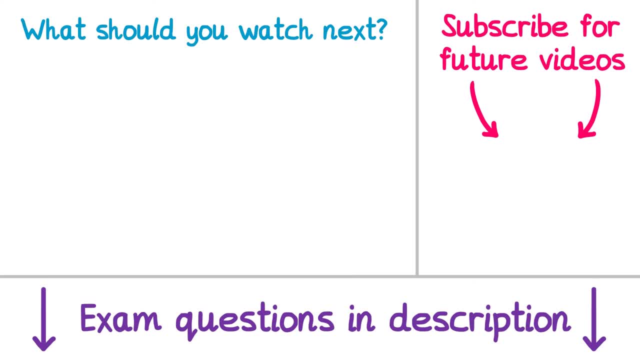 questions that are down in the video's description: what video I think you should watch next and also subscribe, so you don't miss out on future videos. 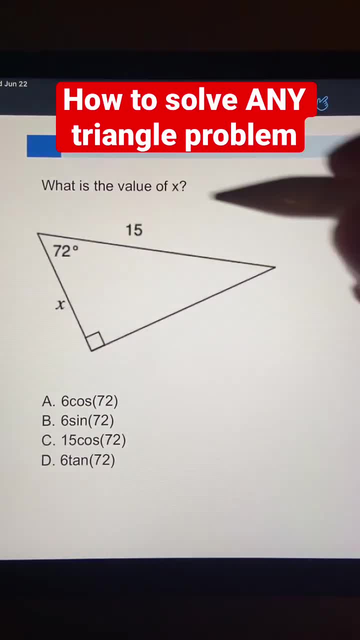 So this problem is asking for this missing side length here, and the first thing you want to do is label all the sides in respect to this angle. So this is going to be the adjacent side, this is going to be the opposite side and this is going to be the hypotenuse. So, if you remember SOHCAHTOA- 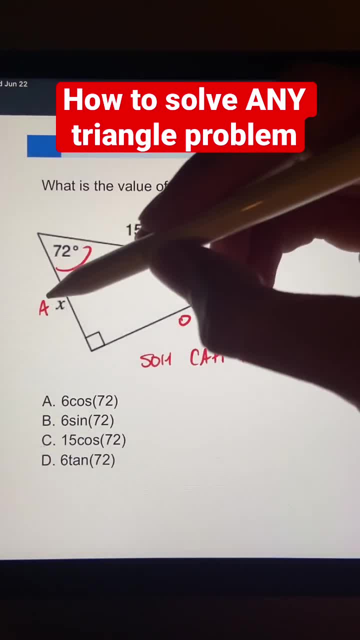 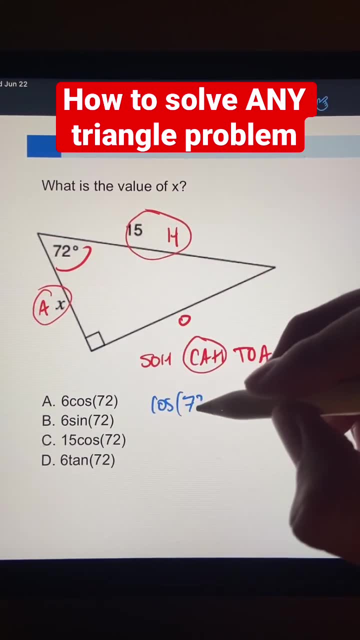 what that tells us is. it tells us what equation we need to use. So we want the adjacent and the hypotenuse. so that means that we have to use cosine. So let's go ahead and write that down here. So cosine of this angle, which is 72, is equal to the adjacent side over the hypotenuse. 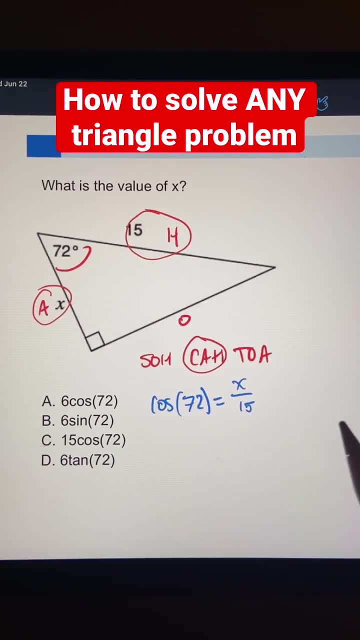 which is going to be x over 15.. So now all we have to do is get x by itself. So let's multiply both sides by 15.. So now we have 15. cosine of 72 is equal to x, which is choice C. 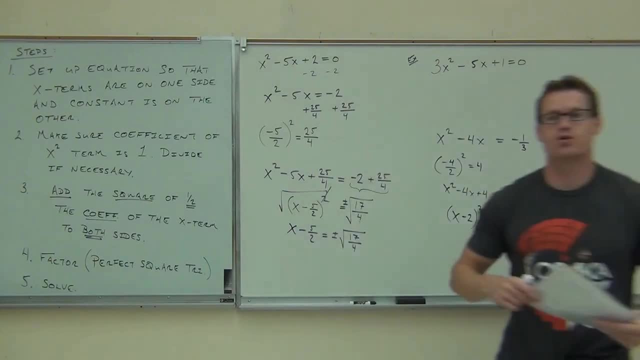 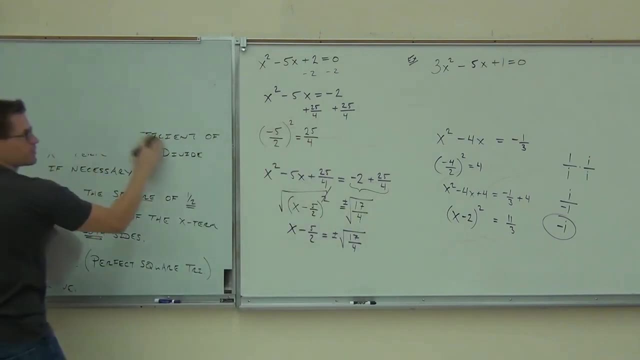 Instead, we're going to learn something in 11.2 called the quadratic formula. However, I'm going to keep one of these on the board because what we're going to do in this example, we're going to solve a quadratic equation once and for all, which means we're going to do it universally and thereby create a formula you can use all the time that works just to the coefficients. It's a pretty awesome idea. Do you agree that any quadratic equation can be written as a? AX squared plus BX plus C equals 0. 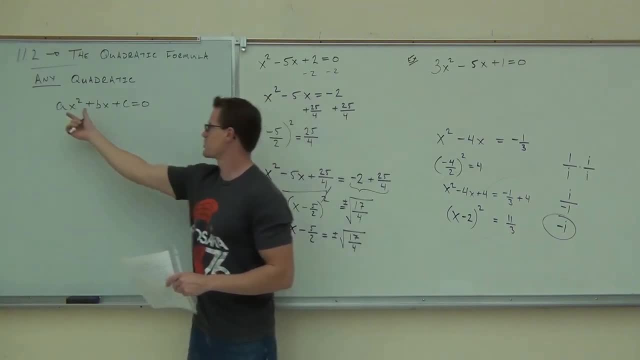 Do you agree that any quadratic can be written that way? This has an X squared term, an X term, and a constant. 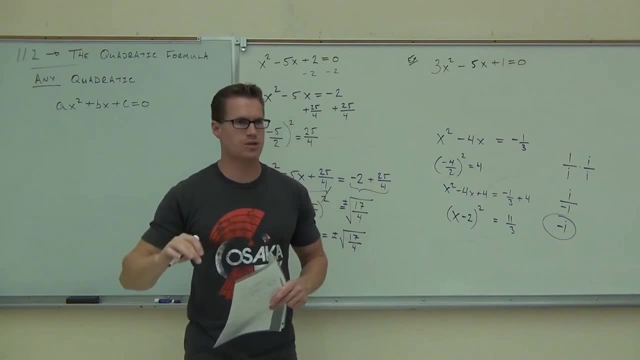 Everything can be written off to one side and 0 on the other side. Are you with me still? 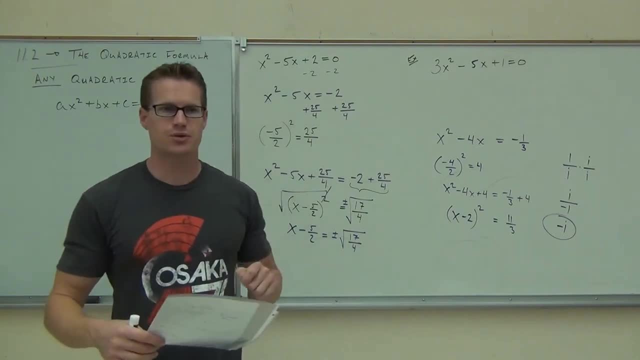 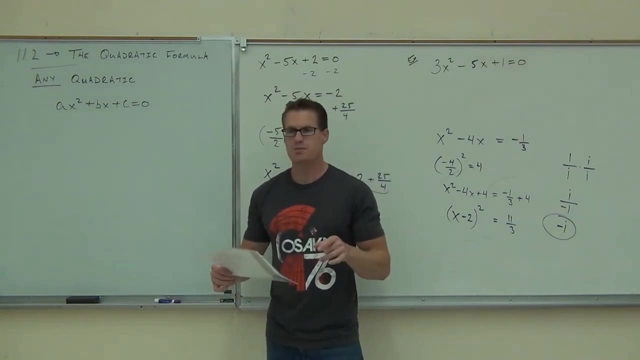 What we're going to do is we're going to use completing the square to create a formula. I'm going to show you the process. What I want you to do right now, if you'd like to, take notes on this, but really, I just want you following. You'll never have to show me this.